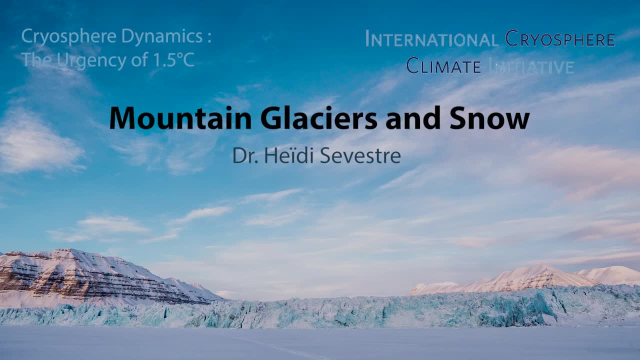 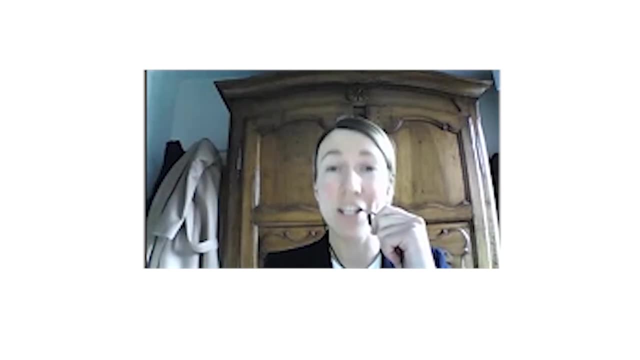 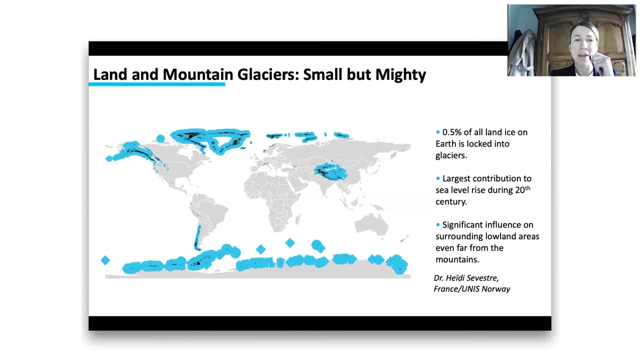 So today I would like to highlight the importance of glaciers for society. Even though glaciers are smaller than our ice sheets, glaciers actually were the largest contributors to sea level rise during the 20th century. If you look at the map on the left, the black. 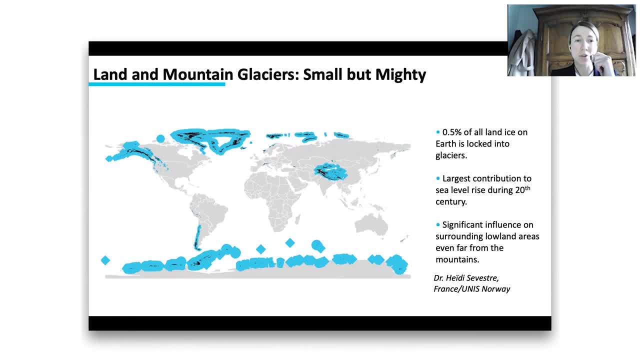 patches delineate glaciers all over the world, while blue areas of different sizes show the potential contribution of these glaciers to sea level rise. Today, all over the world, glaciers are melting and this mass loss is very much accelerating. While the largest glaciers can contribute significantly to sea level rise, the smallest ones, the ones 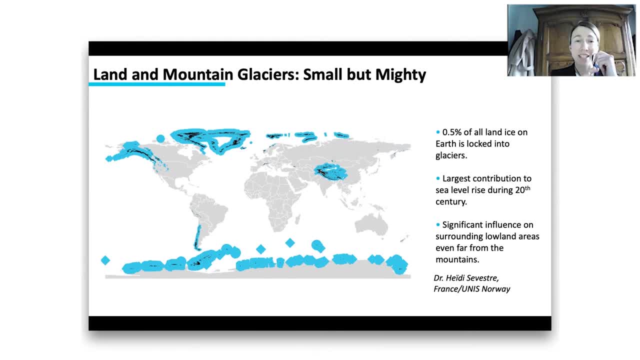 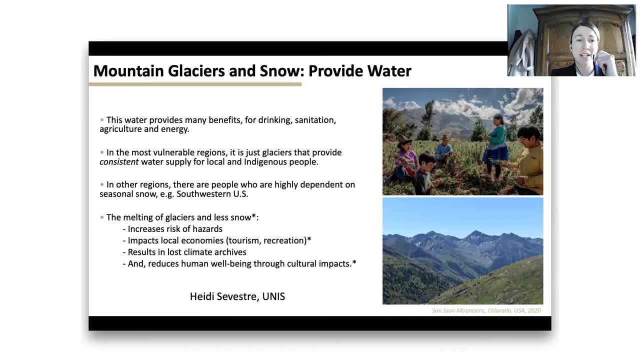 you can barely see on the map, are actually the ones which have the most significant influence on human populations in terms of water supply. So I will now include snow to this presentation, as glaciers are the largest contributors to sea level rise. Glaciers and snow often play similar roles for populations and ecosystems. The main 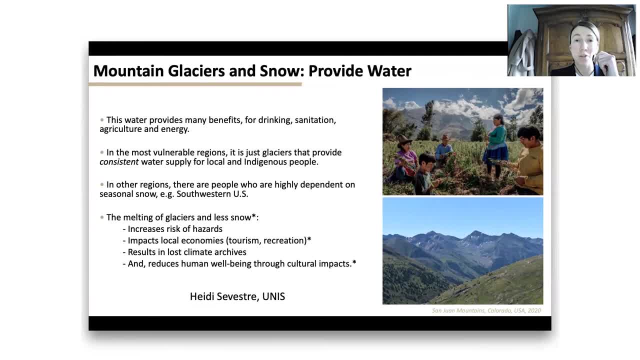 service provided by snow and ice is to provide fresh water when they melt partially or totally. This water can be used for drinking, for sanitation, irrigation, for the production of hydroelectricity. In some regions, like in tropical areas and in the northern Andes, glaciers are the only. 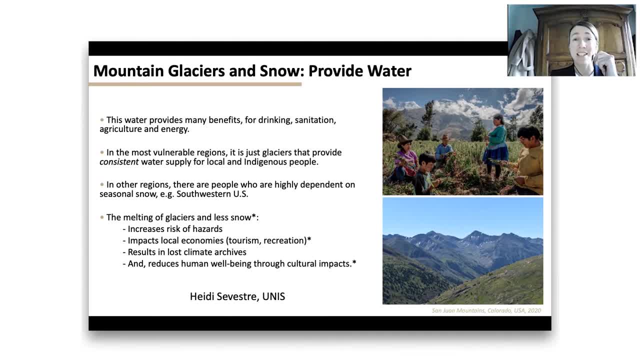 consistent and reliable water supply for local and indigenous people In other regions. sea level rise is the most significant contribution to sea level rise. So if you look at the glaciers, you can see that the seasonal snow is among the most important water resources. 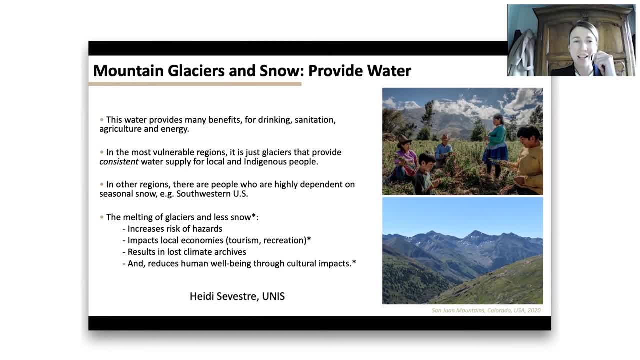 such as in southwestern US, When glaciers melt and less snow falls every year. it leads to a range of impacts, such as a heightened risk of natural hazards, great difficulties for local economies that are connected to recreational winter activities, the loss of climate archives and a reduction in human well-being through cultural impacts. So now we're going to review different geographical areas where glaciers are present. The first one is the Arctic Ocean, which is the most important area of the Arctic Ocean, and the second one is the Arctic Ocean, which is the most important area of the Arctic Ocean. 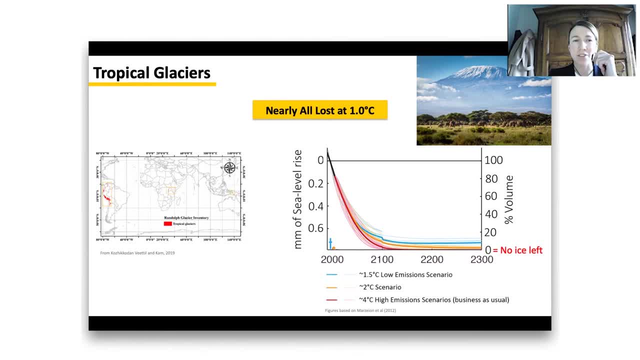 And the third one is the Arctic Ocean, which is the most important area of the Arctic Ocean. We're going to look at all of the regions we have found and investigate projections that have been made for these glaciers up to the year 2300, based on different emission. 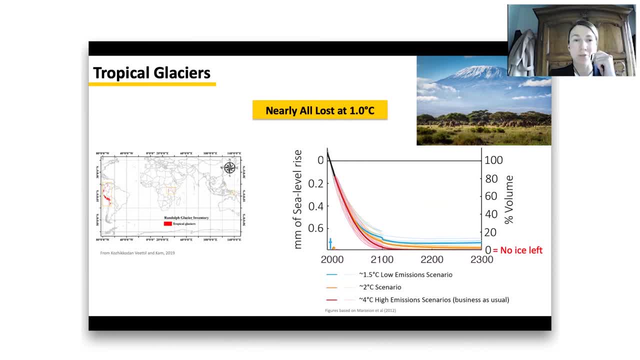 scenarios And we're going to see how much of these glaciers could be left by 2300, depending on the emission scenario we could decide to follow. So in red are the projections for the highest emission scenarios, in orange the middle of the range scenario and in blue 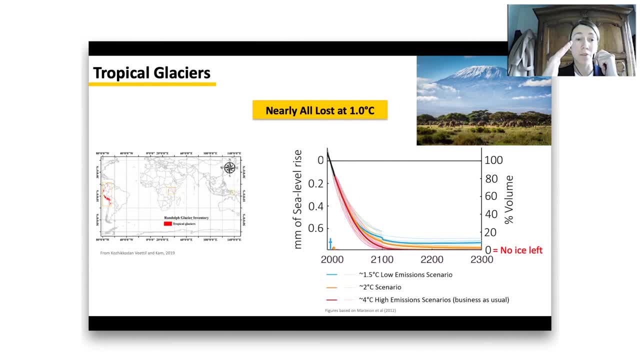 the low emission scenario. When the curves reach the bottom of the award-winning lake, the closest point to the blue lines are the glaciers. So the glaciers that have been left are the ones that have left, And of each graph and the value 0%, it simply means that there is no ice left. So first let's take 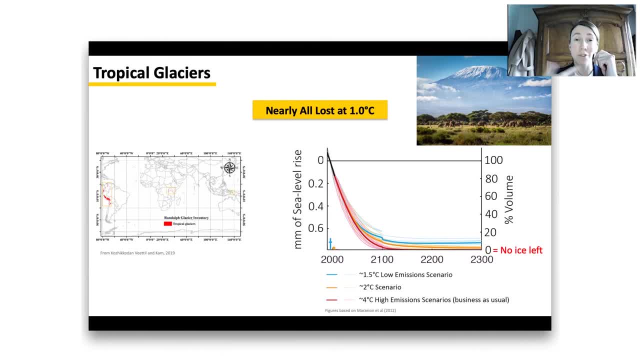 a look at these tropical glaciers. There are still some glaciers left in the northern Andes, in East Africa, in Papua New Guinea. Unfortunately, for most of these glaciers, an increase in temperature of about one degree Celsius is already too much. Very few glaciers will survive beyond. 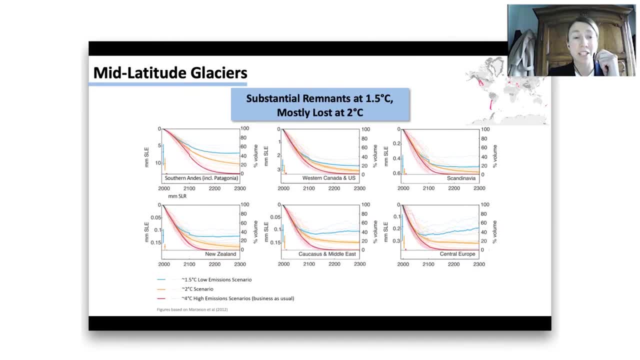 1.5 degrees. So now let's move on to mid-latitude glaciers, where ice loss is also accelerating. In those regions, all of the ice will be gone by 2300 if we keep following the high emission scenario, But fortunately there are other pathways we could decide to follow instead. 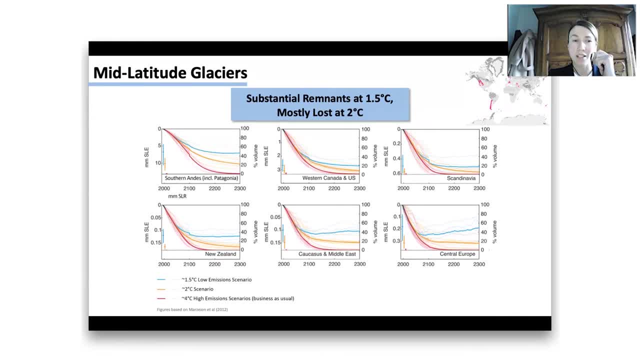 And if global temperatures remain at or below 1.5 degrees, glaciers could preserve up to 40 to 45% of their mass by 2300.. And in central Europe, which is the graph in the lower right corner if you pay attention to the blue curve. 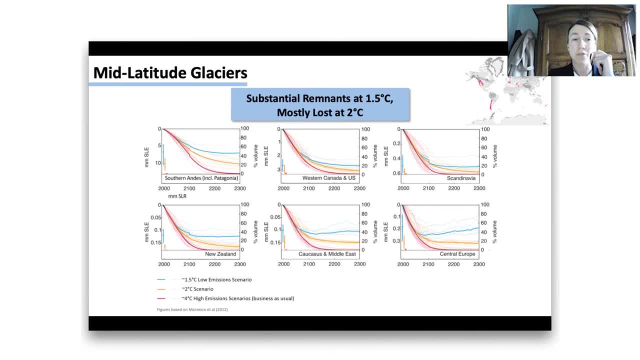 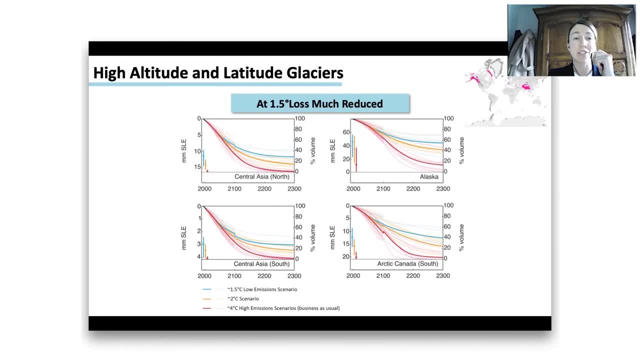 which is a 1.5 degree scenario. we could even get some regrowth of the glaciers, but only if we stay at or below 1.5 degrees. Now let's take a look at high altitude and high latitude glaciers. There again, the differences between pathways are large And, of course, by following 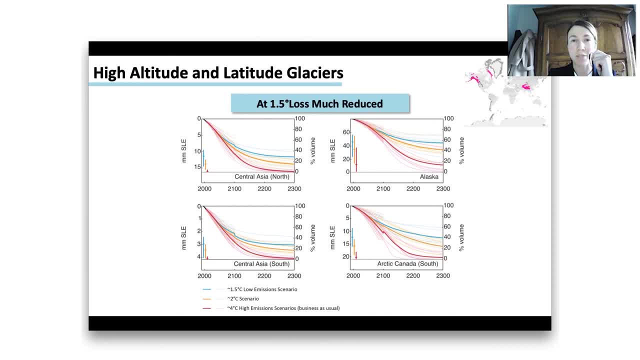 the low emission scenario in blue, we keep much more ice by 2300 than with the other scenarios. It is worth noting that high emission scenarios in red lead to an almost complete loss of ice in the northern and southern parts of Central Asia, where hundreds of millions of people rely on this. 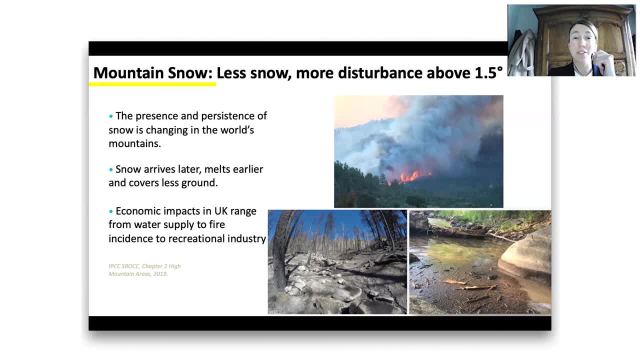 precious water supply. And finally, let's focus on snow. Our current observations reveal that the presence and persistence of snow is changing all over the world. Snow seasons are getting shorter every year and snow covers less ground than before In the UK.